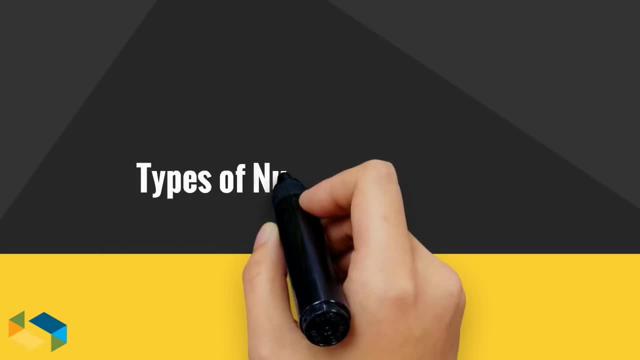 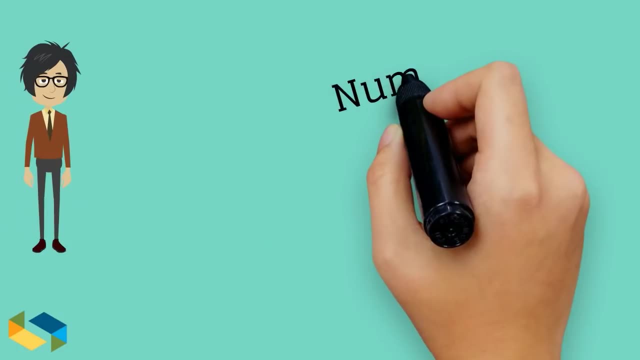 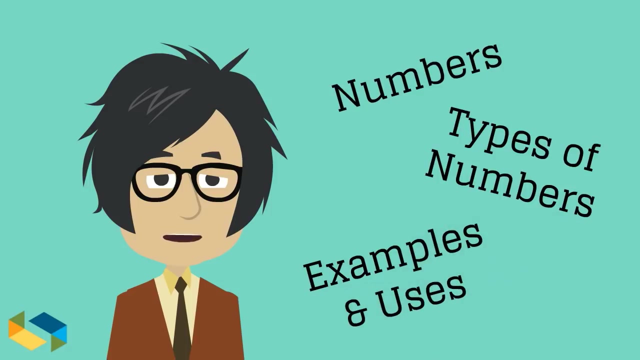 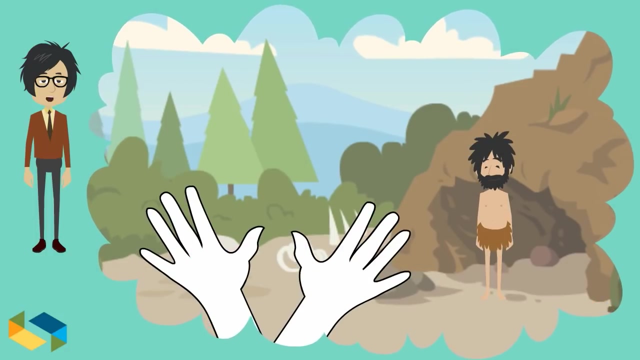 This is the story of numbers, types of numbers, a lot of examples and their uses. So let's jump right in. A long, long time ago, man used his fingers or markings on bones for counting, and later devised various symbols or figures for each number. 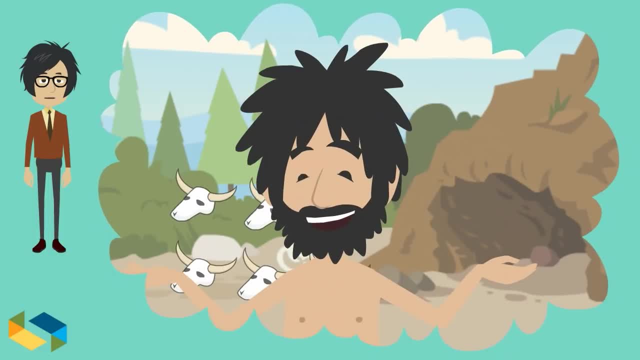 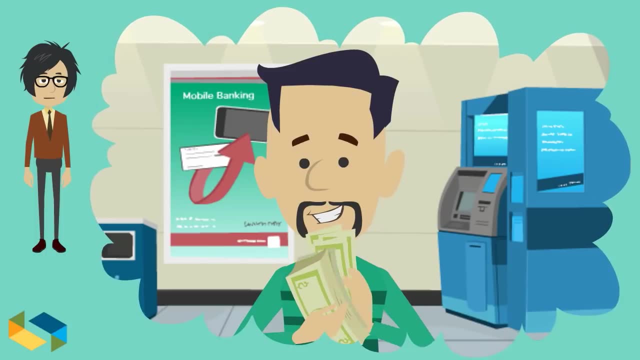 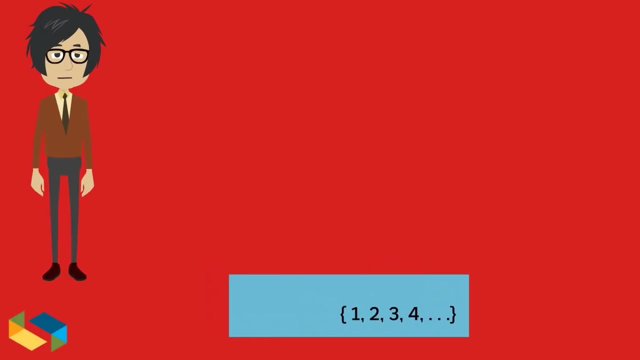 While in those times man normally counted the animals he killed and ate, several thousand years later man is still counting, although mostly money Counting comes naturally to us as something that goes 1,, 2,, 3,, 4 and so on. 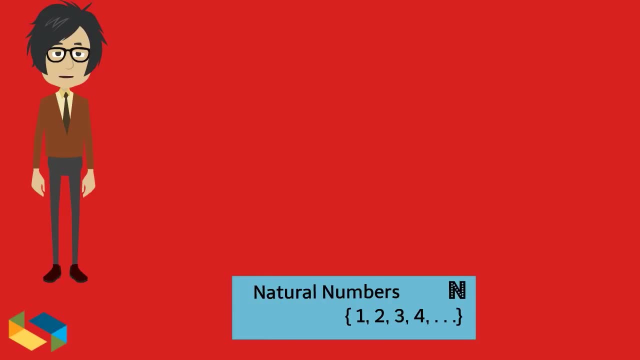 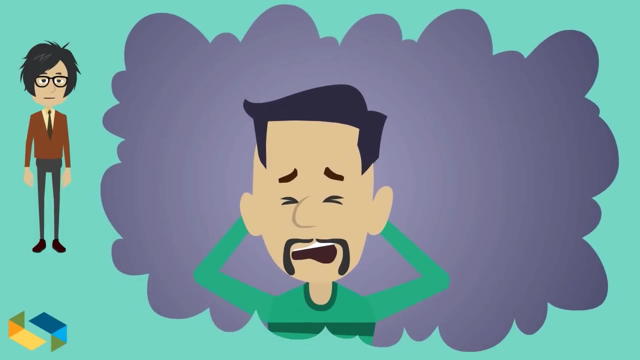 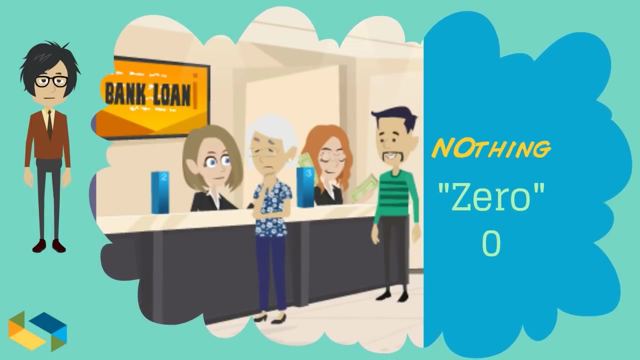 Hence such numbers are grouped as natural numbers with the symbol N. Well, you know, You may be rich one day, but there are days when your flat broke with no money left. So when it comes to describing the notion of nothing, a number zero was discovered. 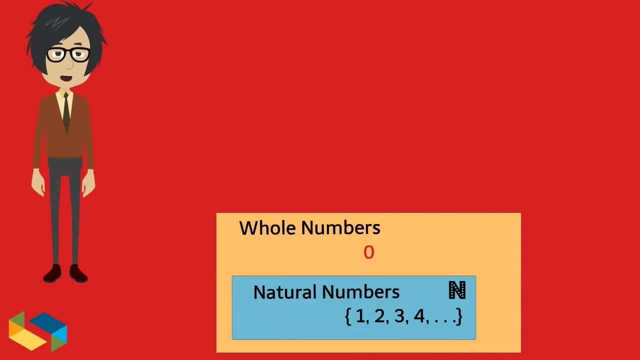 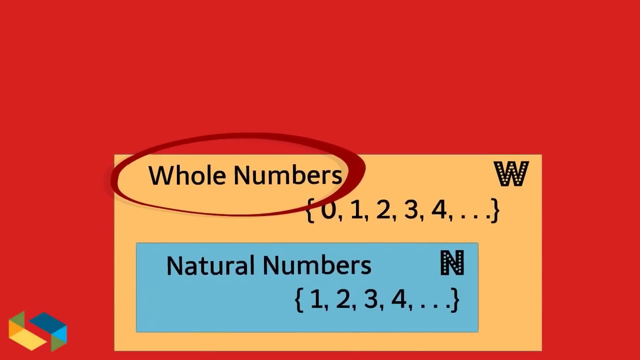 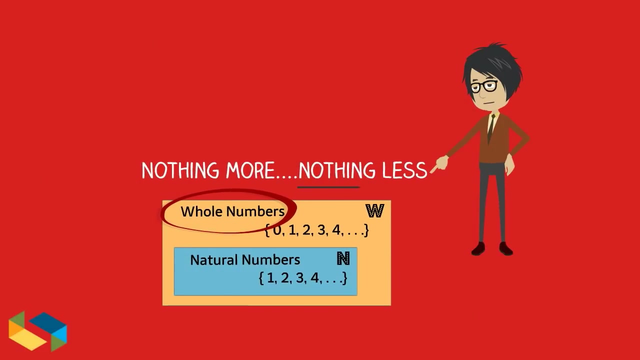 When we add the number zero to the set of natural numbers, we get what is called as the whole numbers, symbol W: In most circumstances, these are the numbers we deal with, Nothing more, nothing less, Except, of course, certain situations prove this to be not true. 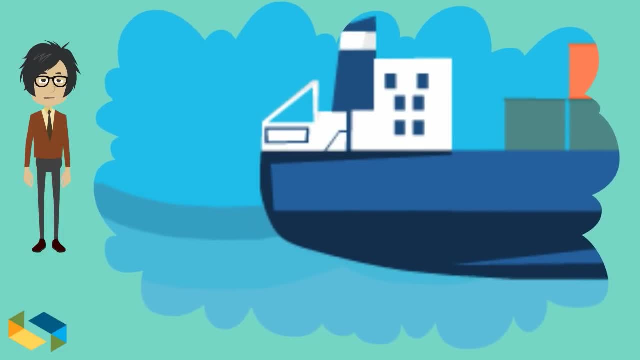 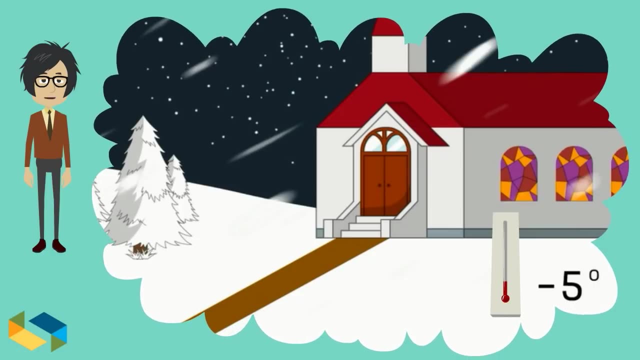 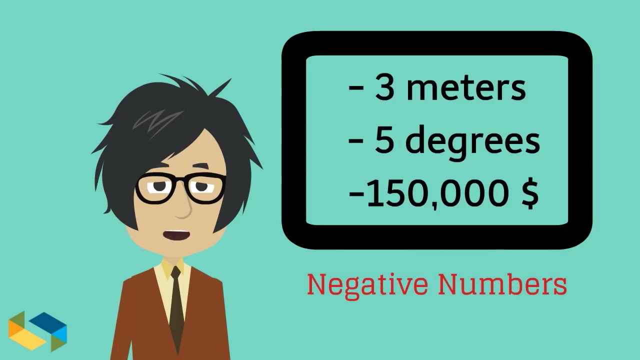 For example, when you have to measure the depth of a ship below sea level, when the temperature drops to sub-zero under very chilly conditions and, of course, when you owe money to the bank. In all such cases, the numbers are called as negative numbers, which, when clubbed together. 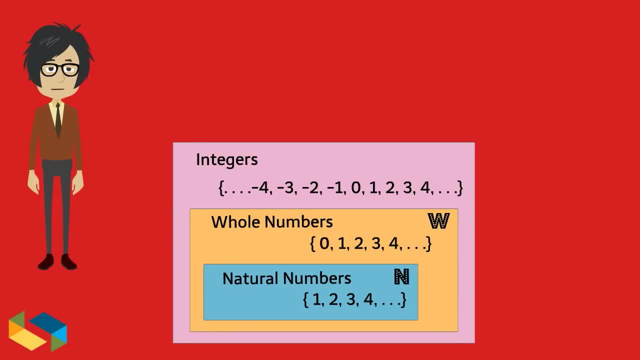 with the whole numbers form a new group called integers, strangely denoted by the letter Z. The term integer has a meaning: It means the number of numbers. In fact, it is derived from the Latin word that means whole, intact or entire. 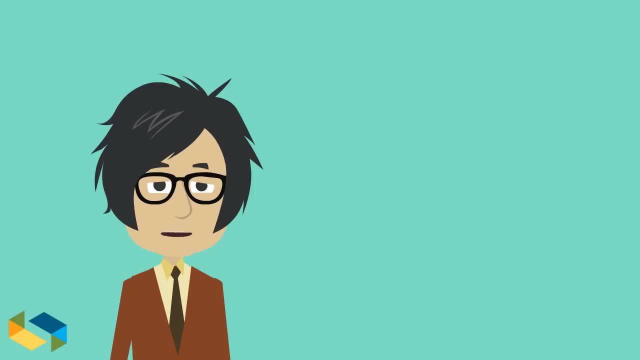 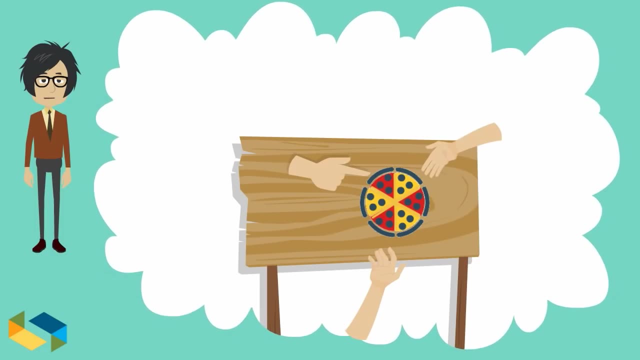 So far, so good. However, there are situations when you are required to deal with parts of a whole, or fractions as they are called, For example, parts of a pizza measuring height more accurately, in this case, 1.5 meters. 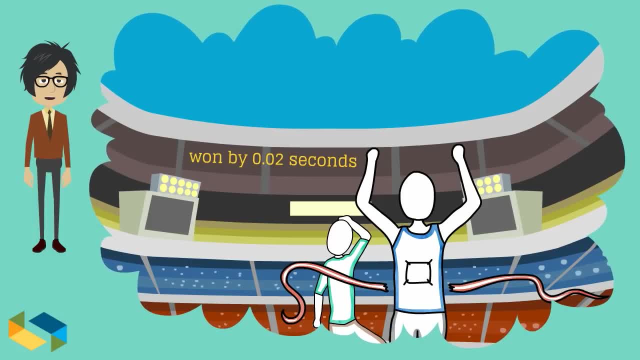 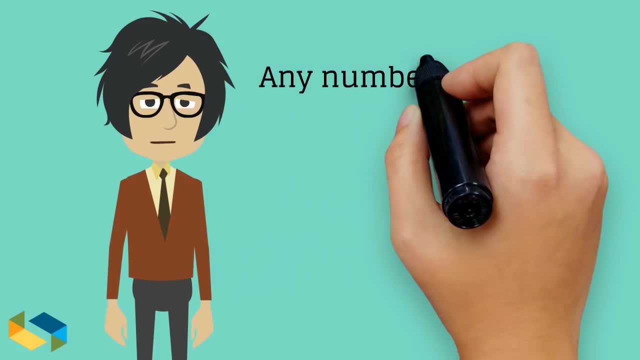 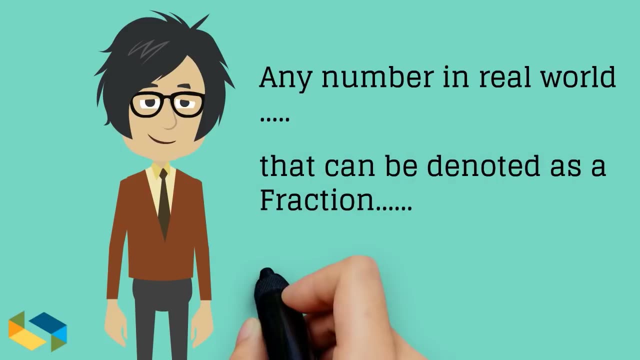 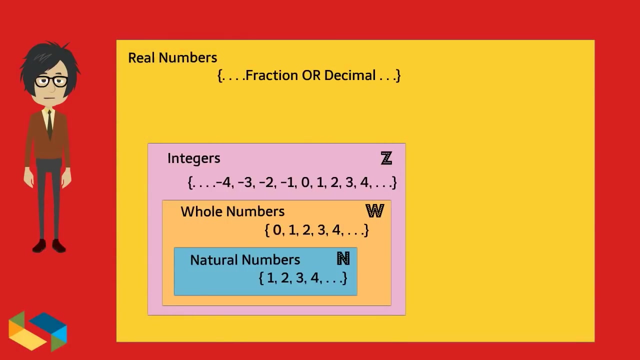 Calculating the fraction of a difference in time in a very, very close race, Specific measures of ingredients in a cake recipe, and so on. So any and every number that you can practically think of in the real world, which can be denoted as a fraction or in a decimal form, constitute what is called as real numbers expressed. 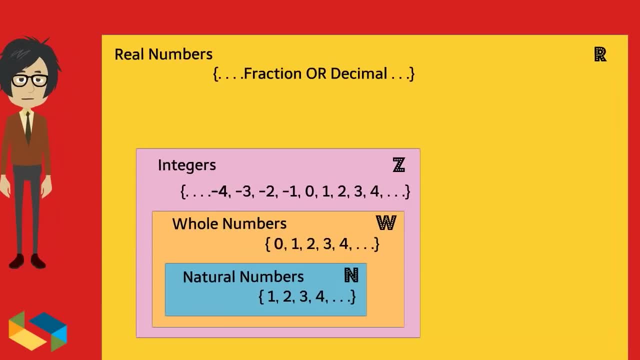 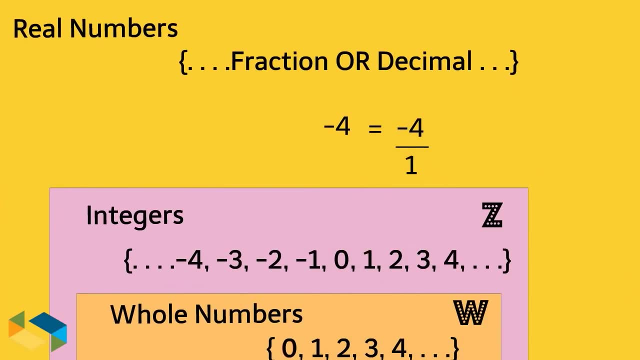 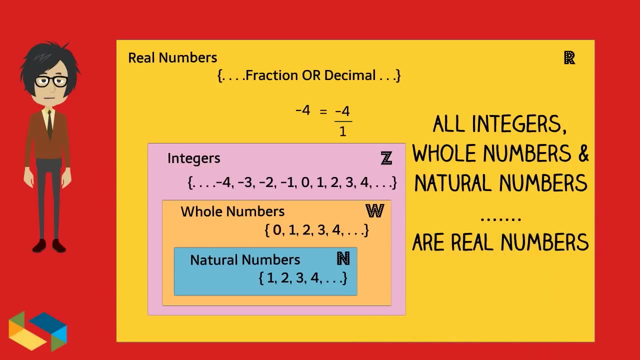 as the symbol R. Now take any integer, say minus 4.. This number can be denoted as a fraction, Namely minus 4 upon 1. So all integers are real numbers too, as obviously are the whole numbers and the natural numbers. 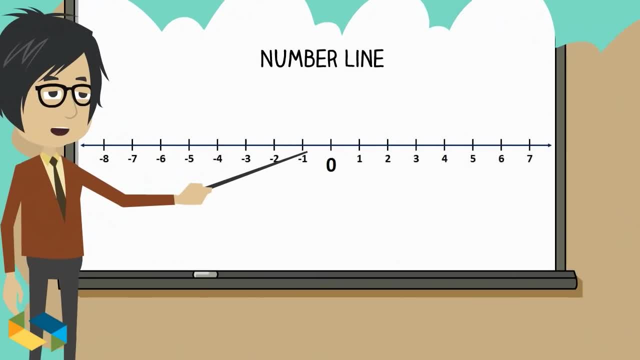 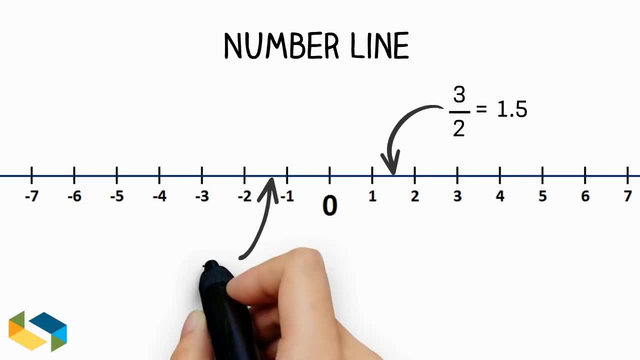 as well. Here are some examples of real numbers. on the number line We have 3 upon 2,, which is 1.5.. Minus 1 upon 3,, which is 0.3333.. Just keep repeating the decimal digits. 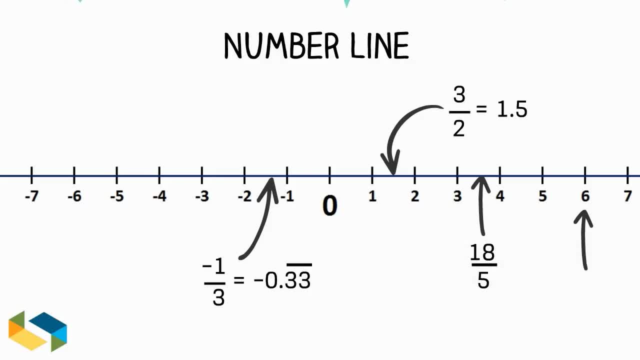 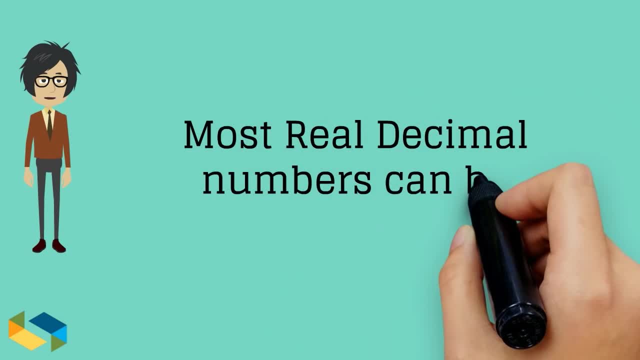 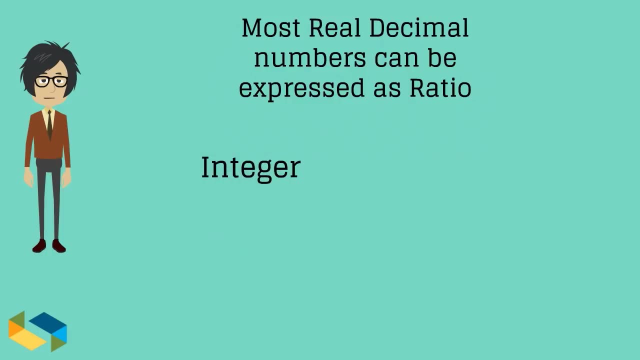 The number 6.. 18 by 5,, etc. etc. Now most of the real decimal numbers can be expressed in the form of a ratio. What I mean by this is that the number can be written as a ratio of two integers. 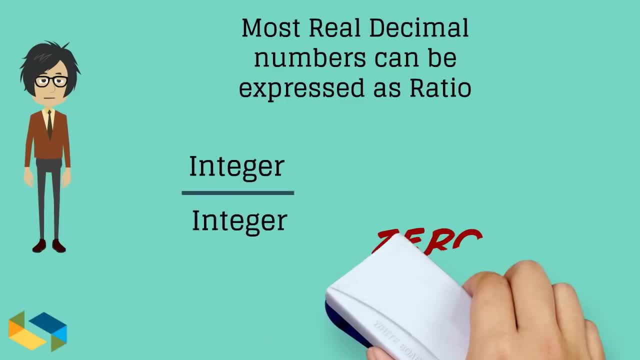 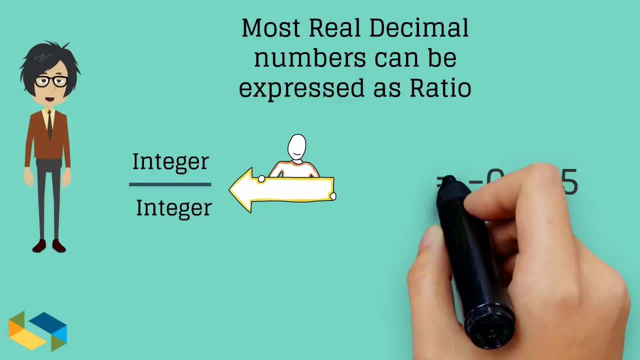 Of course, the denominator cannot be 0.. For example, 0.4 can be written as the ratio 2 upon 5.. The denominator cannot be 0.3.. The denominator cannot be 0.3.. Minus 0.375 is minus 3 upon 8.. 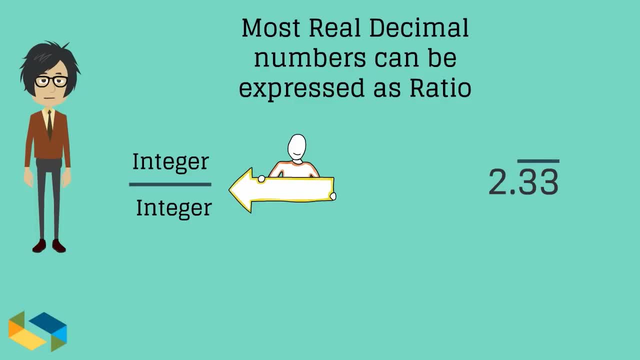 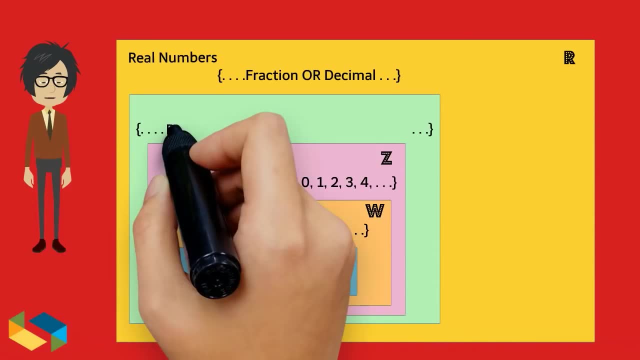 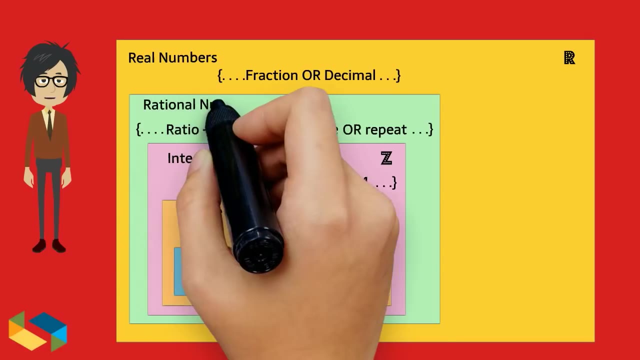 Also 2.33, where the decimal 3 keeps repeating forever, can be expressed as 7 upon 3.. So the numbers that can be expressed as ratio of integers where the decimals terminate or repeat, are called rational numbers. On the other hand, there are some numbers that are irrational.